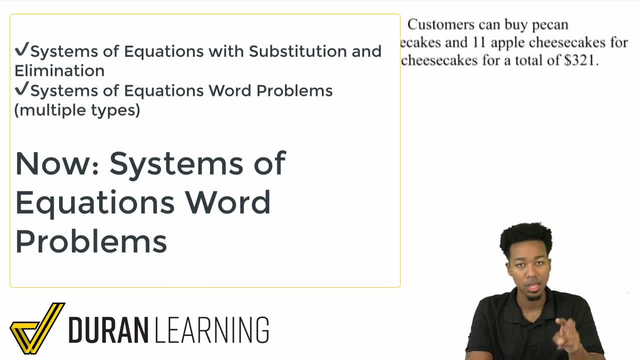 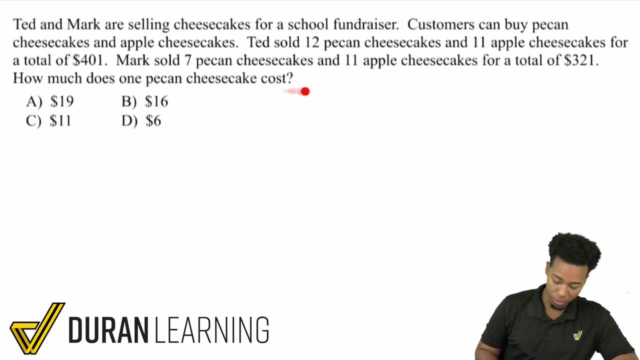 have two relationships about those two things. so for example, in this one here- let's take a look- it says that here you know, what we're looking for is how much does one pecan cheesecake cost? okay, okay, okay, how much does one pecan key cheesecake cost? so I'll go ahead and say here that we'll say P dollars for pecan. 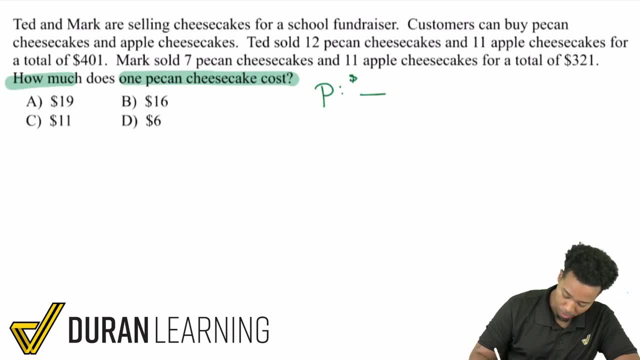 sounds good. so P represents the amount of money that you're going to spend on a piece of cheesecake and P represents blank dollars for one pecan cheesecake. so you may be thinking of this and you're saying: hey, Anderson, we only have one thing that we don't know: what are you talking about? how is this a system? 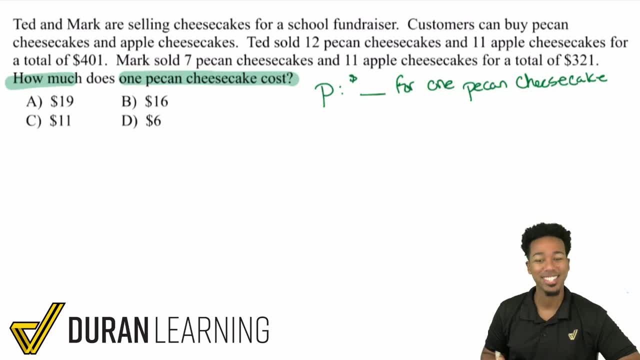 let's take a look at the information. let's break it down so I can show you exactly how this works. so over here, Ted and Mark are selling cheesecakes for a school fundraiser. customers can buy pecan cheesecakes and apple cheesecakes, and then we also have a for apple cheesecakes. do you read this and do you? 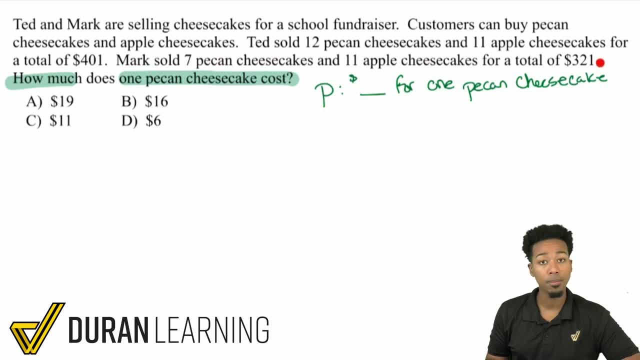 see how much one apple cheesecake cost. no, no, we see the number of them. we see the number of them right over there and there, but I don't see the cost of an apple cheesecake. I didn't even know apple cheesecakes existed. so this is. 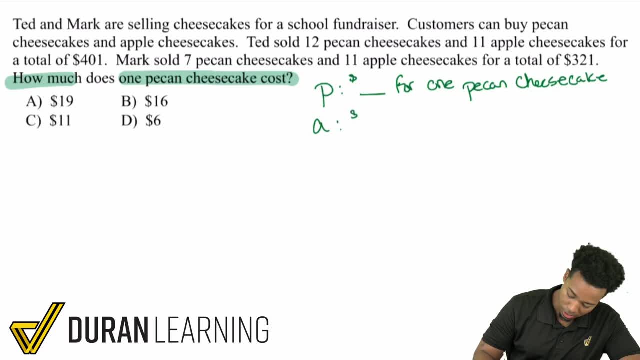 crazy to me, but here I'll just go ahead and say a and that's the cost for one apple cheesecake. so notice, we have two things that we don't know. and look at these two scenarios, look at these two relationships that we have over here. we 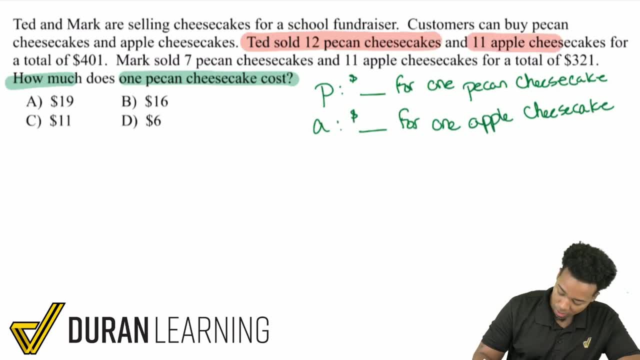 see that Ted sold 12 pecan cheesecakes, 11 apple cheesecakes for a total of four hundred and one dollars. my man can sell cheesecakes, perfect. and then over here on the second end we see that Mark sold seven pecan cheesecakes, 11 apple. 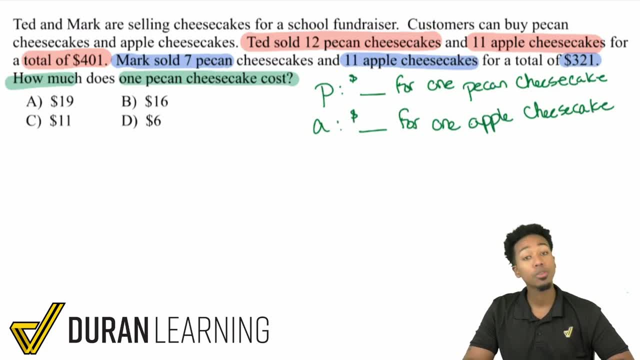 cheesecakes for a total of three hundred and twenty one dollars. so you again, you have two things that you don't know: the cost of a pecan cheesecake and an apple cheesecake. and then you also have two relationships: what Mark sold and what Ted sold. there you go, you're good to go. you have two things in two relationships. 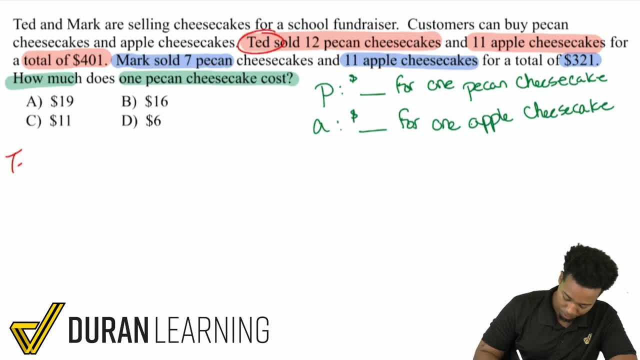 let's set it up. so over here for Ted, let's set up Ted's equation. Ted says he sold 12 kind cheesecakes- pecan cheesecakes, whatever you want to say, however you want to say it, but we have 12 pecan cheesecakes and we know that P. 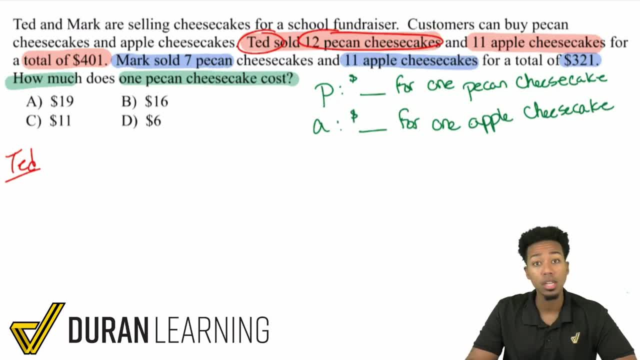 is how much one apple cheesecake costs, those pecan cheesecakes cost. so think about it. if you know how much they cost and you know how many you sold, what do you do with those numbers? to get the num, the, the money that you generated, you multiply. if you know how much they cost and you know how many you sold, multiply that together. 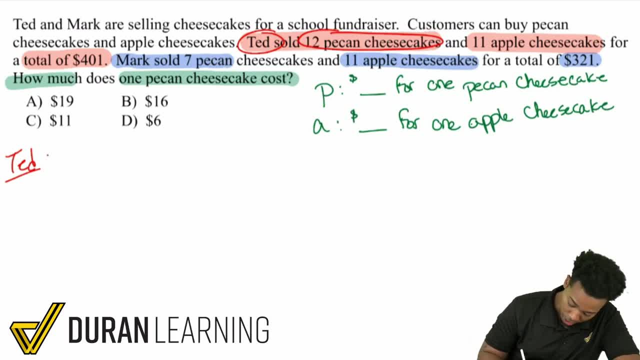 that's going to give you the amount that you earned. so here for ted, that'll be 12 pecan cheesecakes or 12p. then, when it comes to the apple cheesecakes, we have 11 of those and a is the cost of each apple cheesecake. so that'll be plus 11 a, and then from there, when you add up how much you 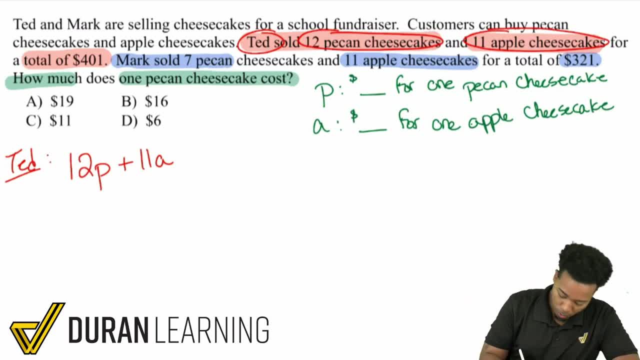 earned from the pecan cheesecakes and the apple cheesecakes. we see that the total was 401 right there. so that's what we have for ted. that's the relationship we can form. now, when it comes to mark, what do we see there for mark? what i see is that he sold seven pecan cheesecakes, 11 apple. 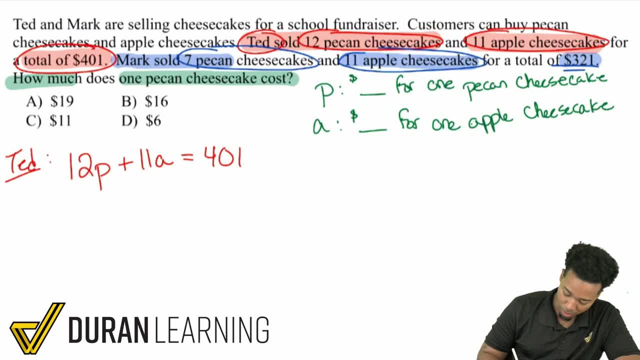 cheesecakes and the total is 321.. so seven pecan cheesecakes would be 7p, 11 apple cheesecakes would be 11 a, and that total would be 321.. booyah, remember my party people. what we're looking for in this problem is p the cost for one pecan. 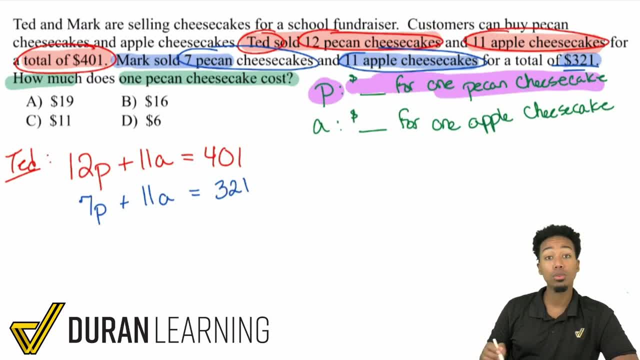 cheesecake. make sure that we remember that. that way you don't get confused and solve for one of the other things accidentally and then think that that's the answer. but now that we have it set up, let's get to work. we have four total problems in this guided practice video, where each of them are: 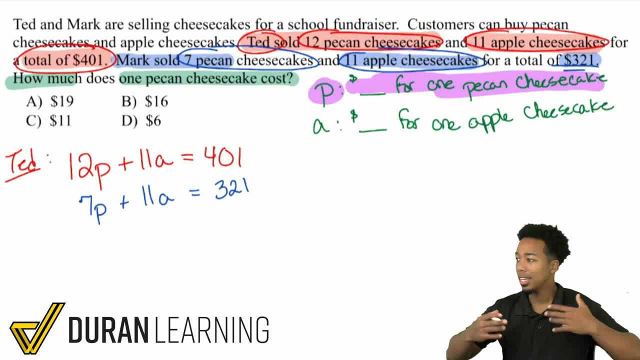 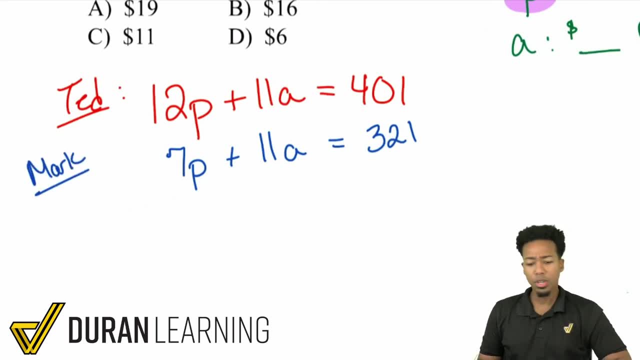 talking about different types of pecan cheesecakes and we're going to go through them one by one, little things, but we're going to be setting them up and again the same fashion. so here, that was ted, this was mark. what can we do here? well, i'm part of people. one thing i: 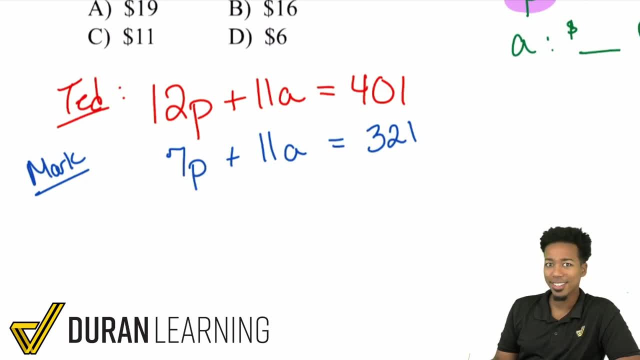 noticed is that hey, uh, i have 11a on both of these. actually, i can actually just subtract the equations because, again, this is a positive 11a, that's a positive 11a. i can just subtract these two equations and i'm good, let's go ahead and get to it here. i'll subtract them and remember we're. 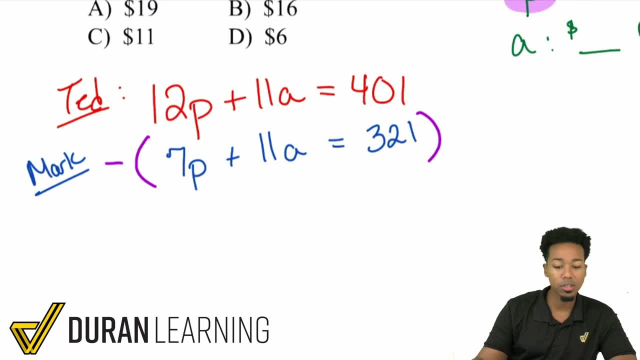 subtracting. so when you're doing this, remember that subtracting is just the same thing as adding the opposite. so what i'll do here is i'll write that we're adding the opposite here. so instead of plus, we write minus. instead of a positive 321, negative 321.. again, subtracting is the same as 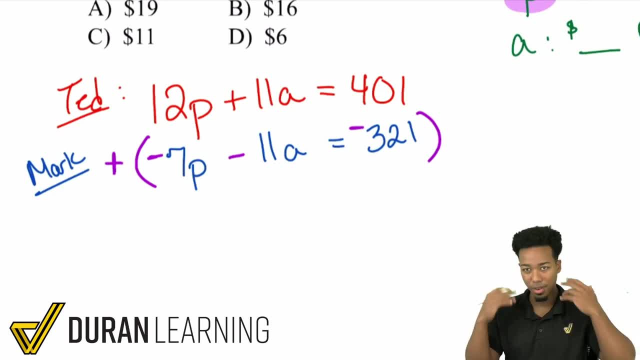 adding the opposite. so we need to be able to do that very quickly and very visually without much trouble. but watch how easy this becomes. now let's go ahead and get to work. if i add these together, what i see that i have is 12 minus 7, and that is 5p. 11 minus 11. boom, those cancel out. 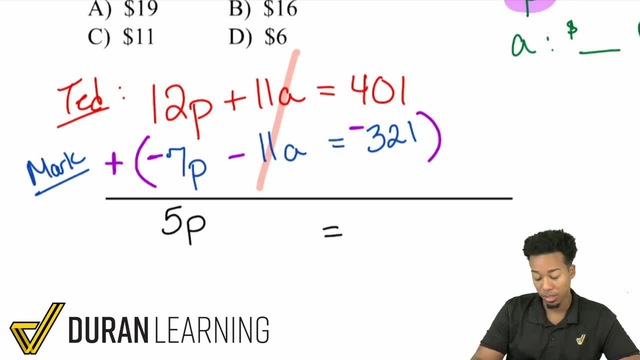 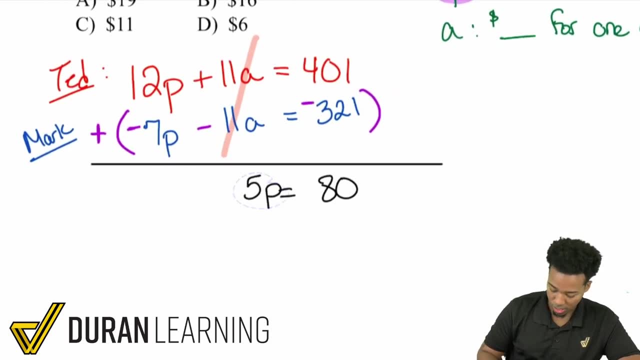 and then 401 minus 321, that becomes 80.. so we have: 5p equals 80.. and so, to solve for p, let me actually just move these together. to solve for p, what we'll do is divide both sides by 5.. 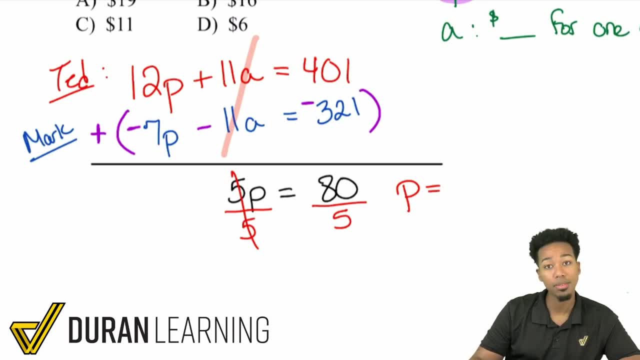 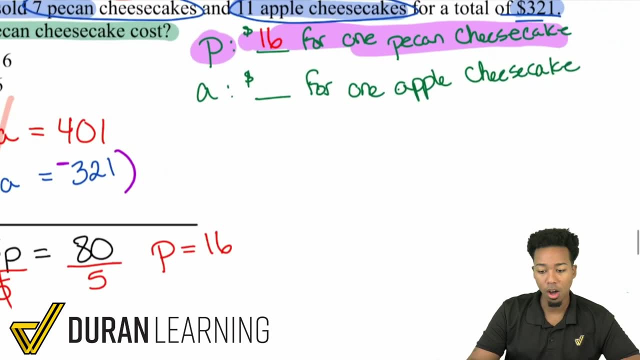 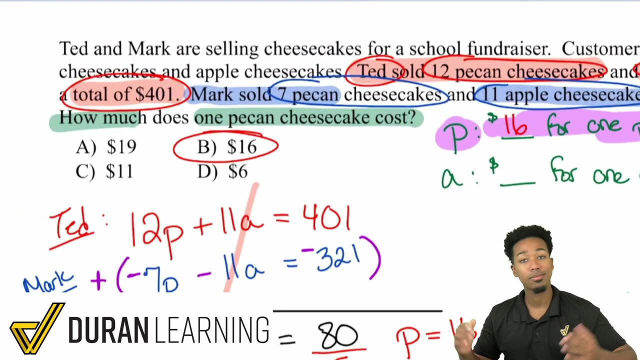 bam, right there. p equals 80 divided by 5, which will be 16.. right there, and so what that means is right here. 16 is the cost for one pecan cheesecake, and that's it. booyah, we have our answer. that's b and we're done now, remember we. 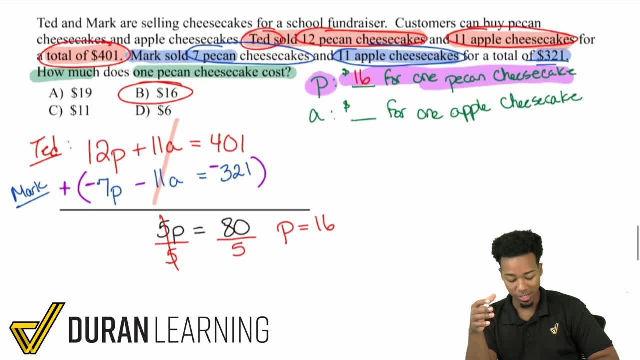 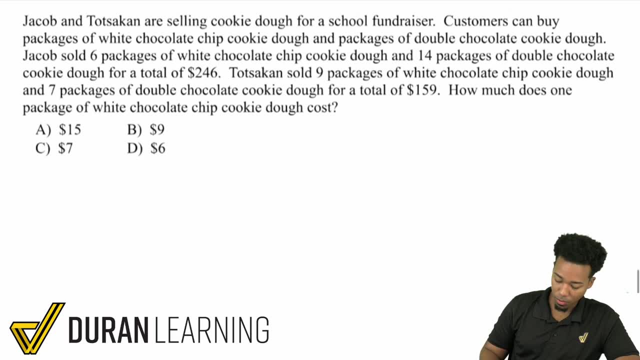 have three more problems here to go, so go ahead and watch through the rest of these, because i got your back here setting these problems up and then solving them. those are the two main things. let's take a look at the next one here. so we have one that looks a little bit. 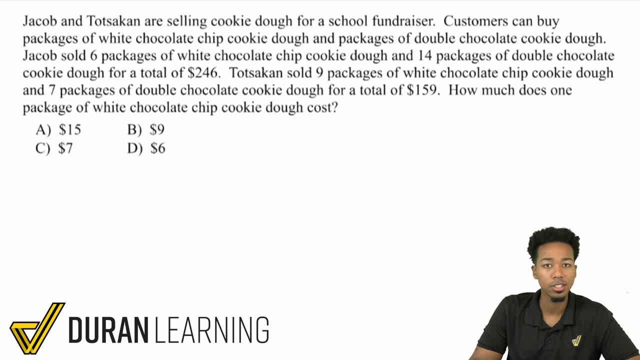 bigger, but don't worry, i don't care how big the problem looks. start with the question over here: how much does one package of white chocolate chip cookie dough cost? start with the question. remember, it's about first knowing what you want, then establishing what you have and then making a connection. that's how we handle word problems. 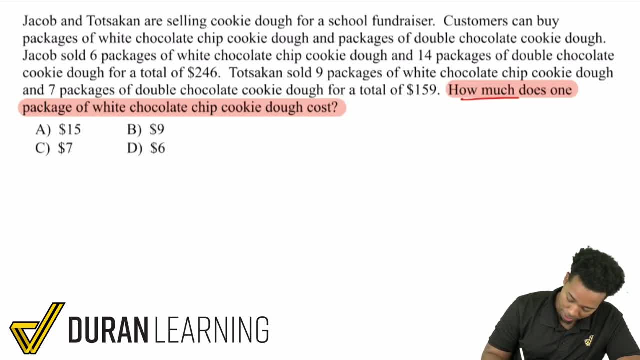 so right over there, how much one package of white chocolate chip cookie dough? so right over here i'll just say w is the cost for one package of white chocolate chip cookie dough. for one white chocolate, all right, cool. now let's go ahead and take a look at the information that's given to us. 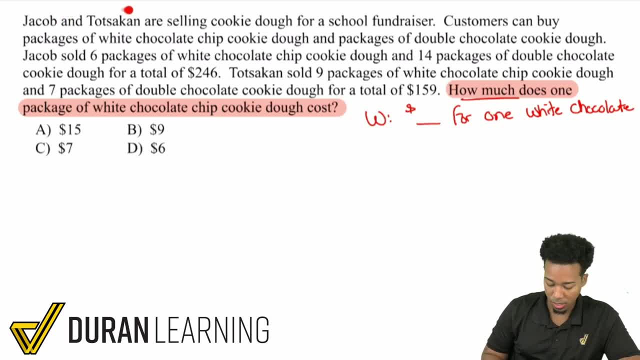 this is how we're going to sort through it. here we go. jacob and totsakan are selling cookie dough for a school fundraiser. customers can buy packages of white chocolate chip cookie dough and packages of double chocolate cookie dough- double chocolate cookie dough- okay. so jacob sold. 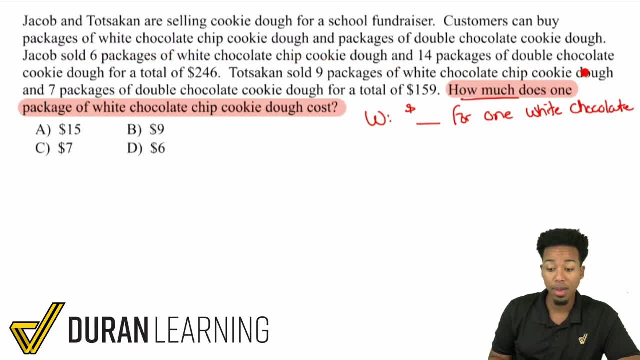 sold six packages of white chocolate chip cookie dough and 14 packages of double chocolate cookie dough for a total of $2.46.. Toksakun sold nine packages of white chocolate chip cookie dough and seven packages of double chocolate cookie dough for a total of $1.59. 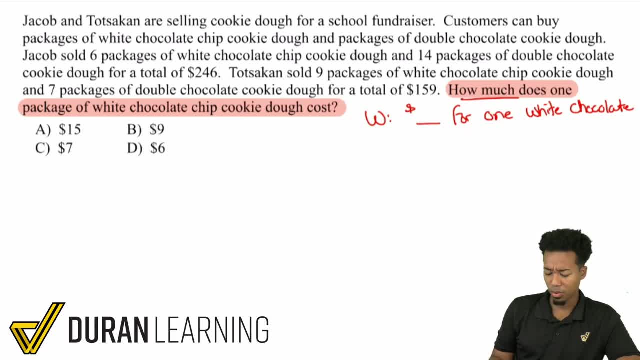 So what am I looking at here? I know that one variable that I know I'm looking for is again the cost for the white chocolate, but I keep seeing them mention the double chocolate, which I don't know, And that's what I'm going to have to write down. 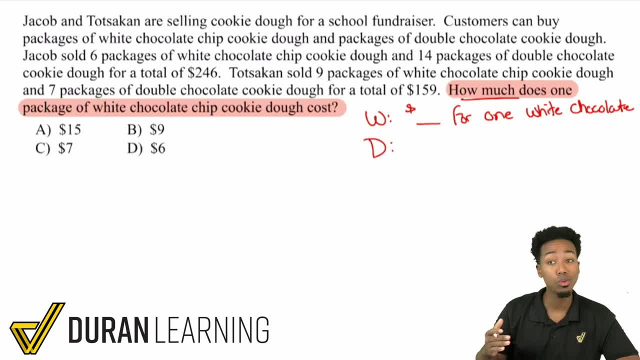 I got to make sure to write that down as well, because that's going to be useful, because it's included in both relationships. So I'll just say D is the cost for one double chocolate. And before we continue, my math party people really quick. before we continue, I know that. 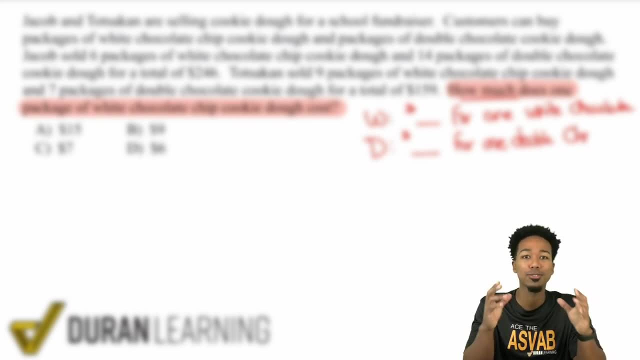 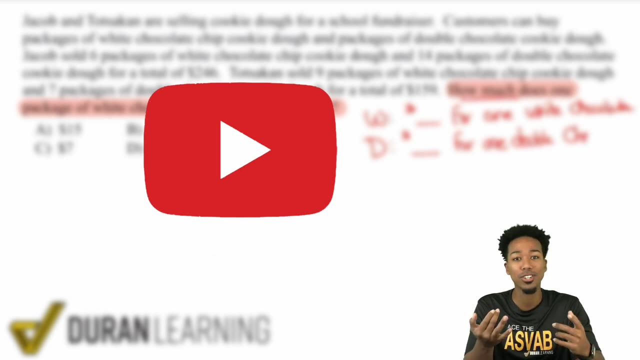 you're enjoying this video and I want to make sure that more people can enjoy these videos, just like you. So, if you wouldn't mind, just take a quick second, like this video, comment on it, just showing some appreciation, showing what you learned, and then make sure you're subscribed. 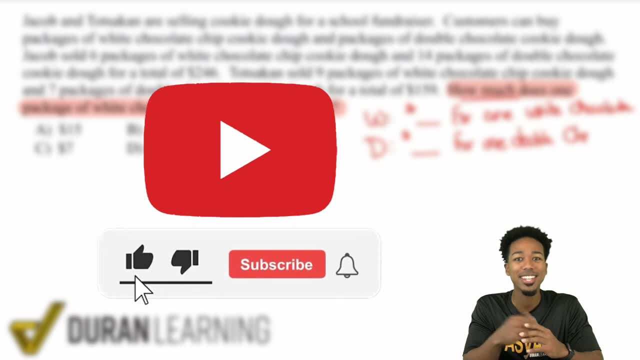 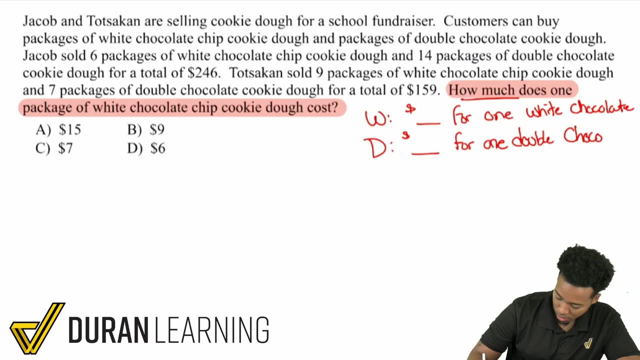 to the channel, So that way, when we come out with new videos, typically every day, you can be right there on the spot to catch on to them. So help us, help others. ace the ads. babe, I'm Anderson, Let's keep going here. 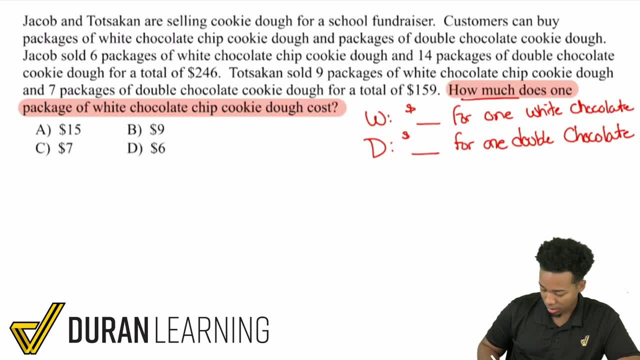 And I write that right there. So I have W and I have D, but I need to continuously remind myself that I am looking for W. Just keep that in mind. But I have two things that I don't know. but remember that you're looking for W And so 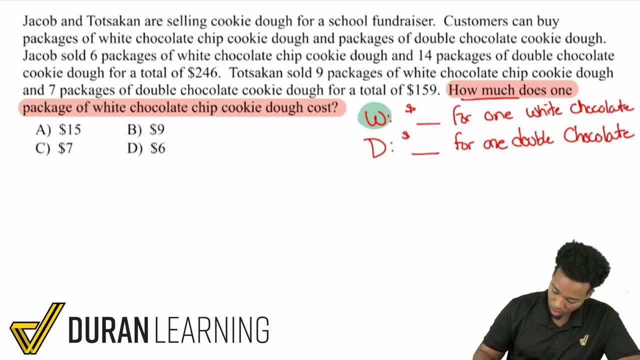 let's go ahead and set this up here. We see, right here, right over here, Jacob sold someone. highlight this in blue. Jacob sold six packages of white chocolate chocolate chip cookie dough, 14 packages of double chocolate chip cookie dough. total 246.. 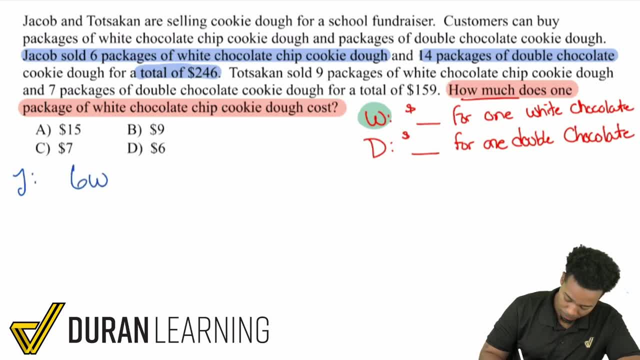 So right here for Jacob, we have six packages of white chocolate chip cookie dough plus 14 packages of double chocolate, and that ended up being 246.. Right there, Because, again to get the total amount of money that you made from the white chocolate. 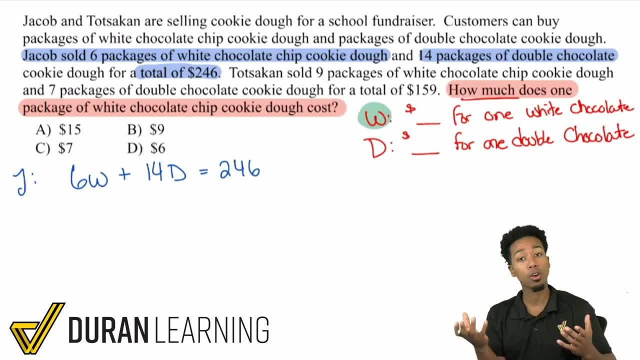 you do W times six, because it's six packages, each of them costing W. I don't know what the number is, but they each cost this much. You multiply to get that total. Multiply the 14 and the D to get the double chocolate. then add it all together to get. 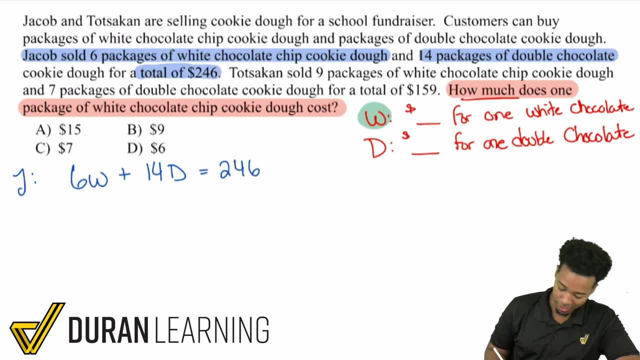 246.. And so from here, let's go ahead and take a look at Toxicon. here I'm going to go ahead and grab green Toxicon. sold nine packages of white chocolate, seven packages of double chocolate total 159.. 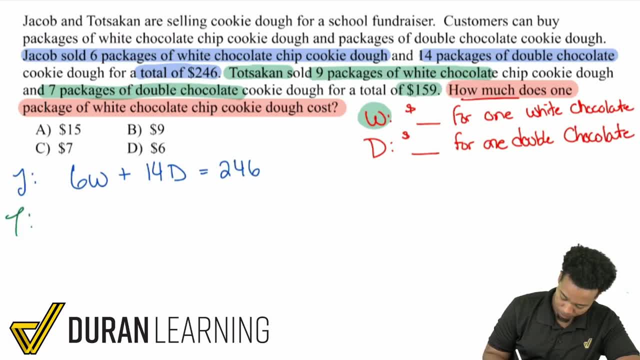 So write that down. So for Toxicon right over here, nine packages of white chocolate plus seven packages of double chocolate, So the total is 159.. And check out this right here. So now that we've set it up, my part of people remember we're looking for W, And if I look, 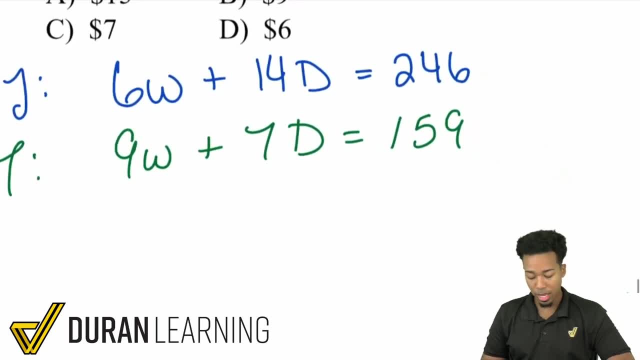 at this. this is pretty interesting because what I can do is I see that we have 14 D and 70. I can actually turn one into the other. I can use elimination here by modifying one of the equations to get the other variable lined up. 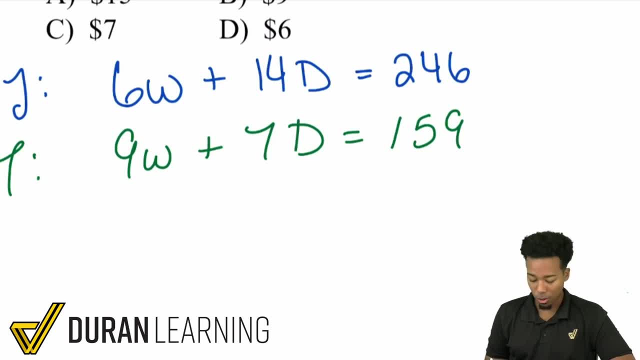 So, with that said, what I'll do here, my part of people is: I'll go ahead and You have. You have options here. You can divide the top one by two or you can multiply the bottom one by two. You can divide the top one by two because 14 divided by two is seven, and all of these. 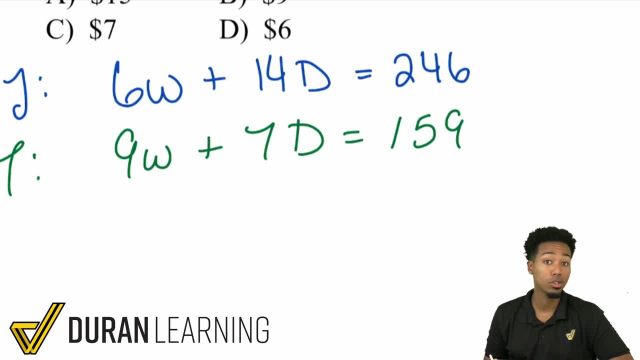 are even So, if you wanted to deal with smaller numbers, you absolutely could, And you know what I'm actually going to do that because in the previous video I had one of the same options, but I chose to multiply instead. But I'm going to show you how to get this done again in the easiest way possible. 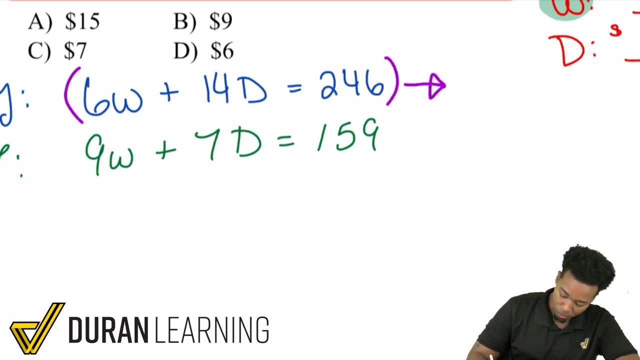 So I'm going to take this entire equation and I'm going to divide the entire equation by negative two. I'm going to divide it by negative two. The reason I'm dividing by a negative is so that I can make this a negative and this a 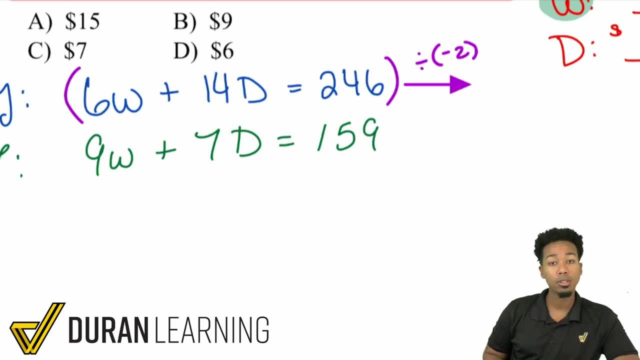 positive. That way we can cancel things out. And I'm dividing by two, because it's going to turn the 14 into a seven, which would line the D's up to cancel out. So, with that said, here we go What I'm going to have. once I do that, I'm going to give myself a little more space. 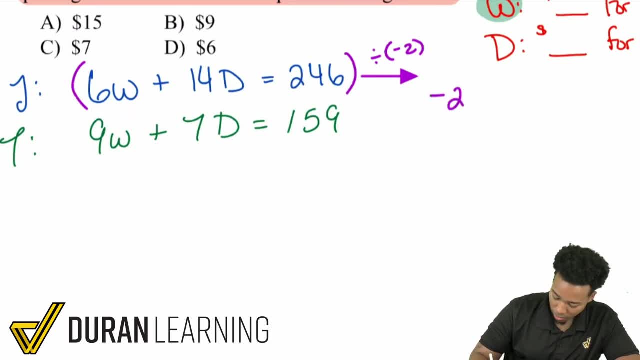 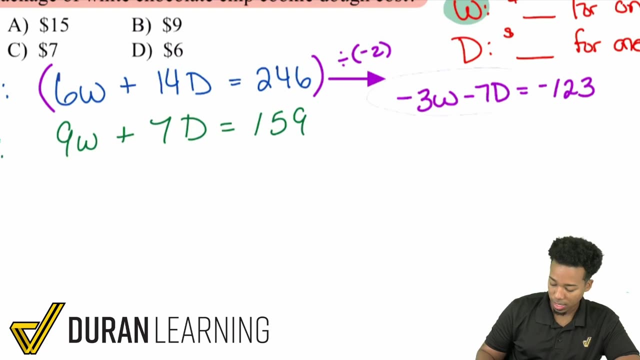 Six W divided by negative two is negative two or negative three W, excuse me there. Then we have 14 D divided by negative two. so that's minus seven D. 246 divided by negative two would be negative 123.. So if I take this and I put it right under here, look at what I can do now. 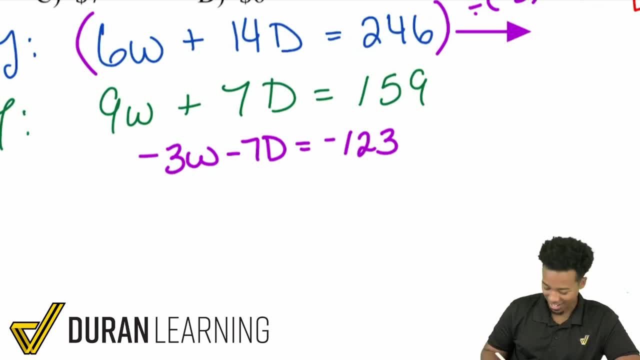 Look at how it lines up. I can add these together and I can cancel it out. So bam, line it up right here. Nine W minus three W, that's going to be six W Over here. the seven D minus seven D that. 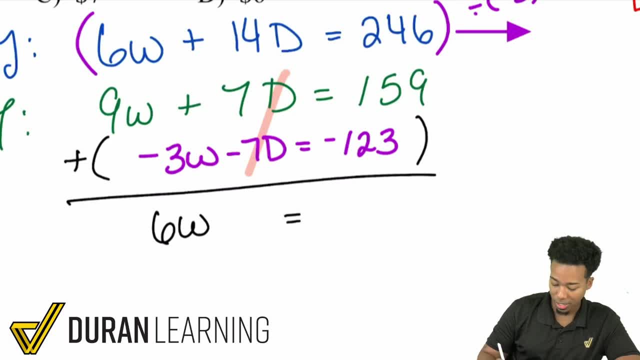 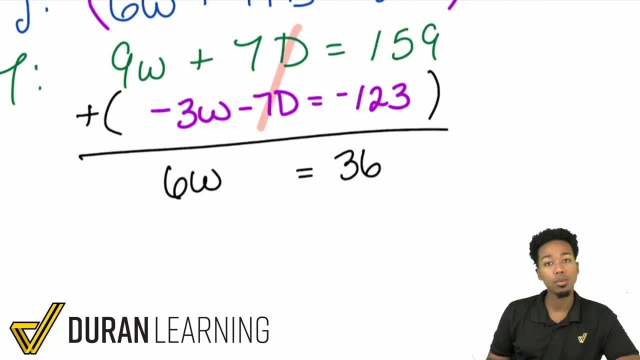 cancels out, And then we have 159 minus 123.. That's going to end up giving me 36.. Boo, yeah. So now we have six W equals 36.. Look at that. I can go ahead and divide both sides by six and look at how much easier this can be if. 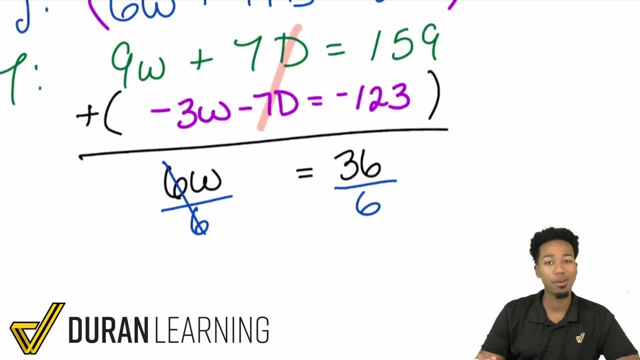 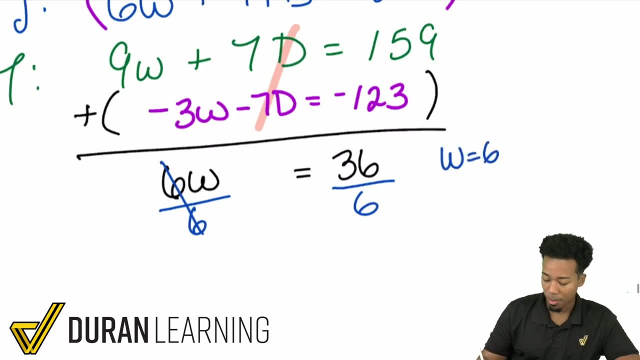 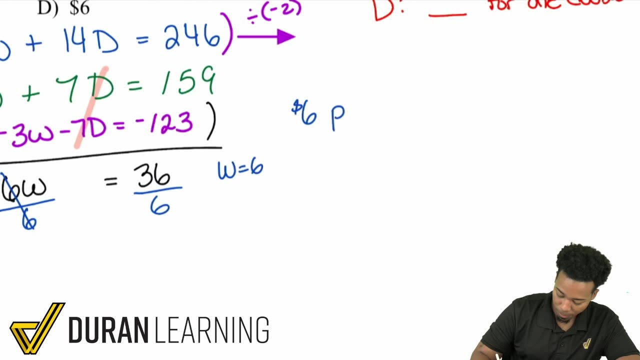 I divided that top equation instead of multiplying the bottom one and getting huge, way bigger numbers, And so here W equals six after I divide. And remember what W represents is the cost for one white chocolate chip package. So that means that it's $6 per white right over here. let me go ahead and fix that. 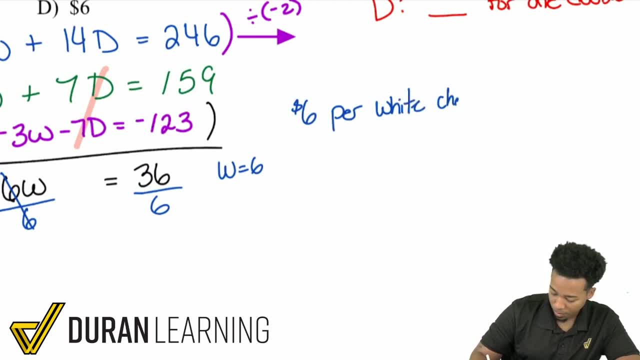 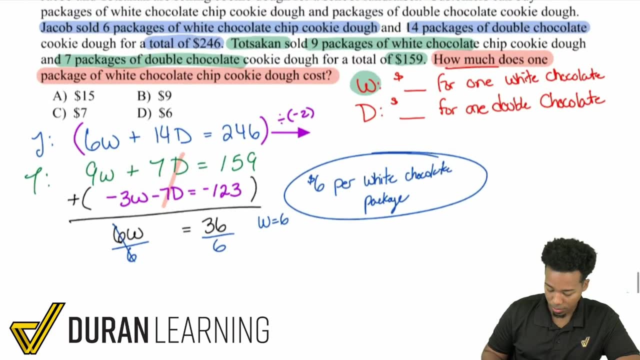 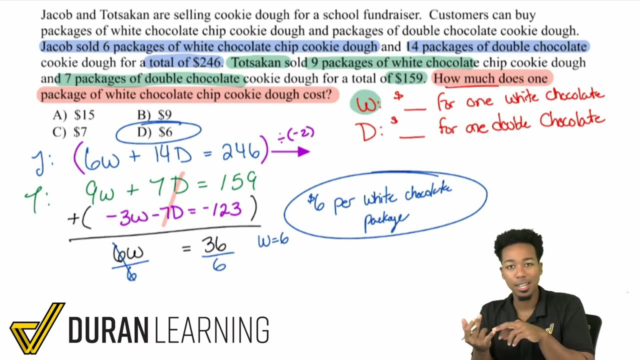 There we go For one per white chocolate package, booyah. And so we have our answer: It's $6 per package, That is D, and we're done. And so again my math party people look, setting it up is just as important as solving. 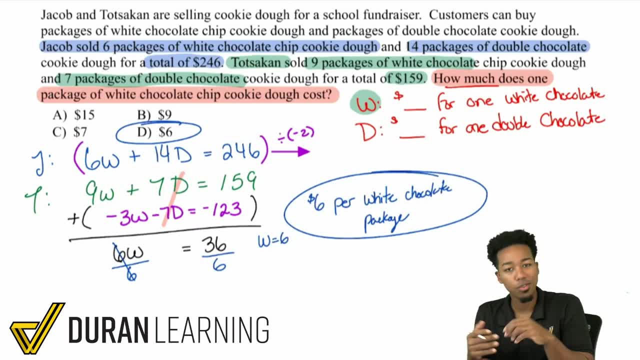 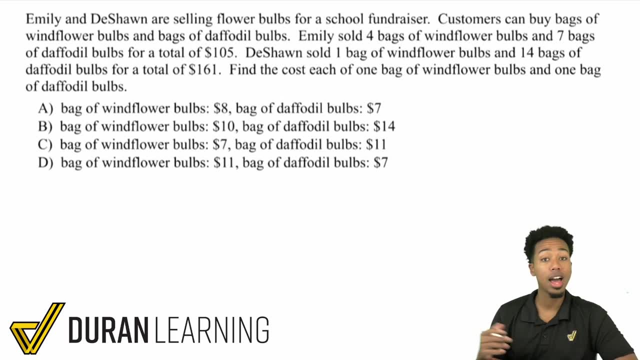 We need to know how to set it up. So, with that said, let's go over another practice problem. here We got this. Here's another one. Let's talk about Emily and Sean. They're talking about selling flower bulbs. Sounds good. 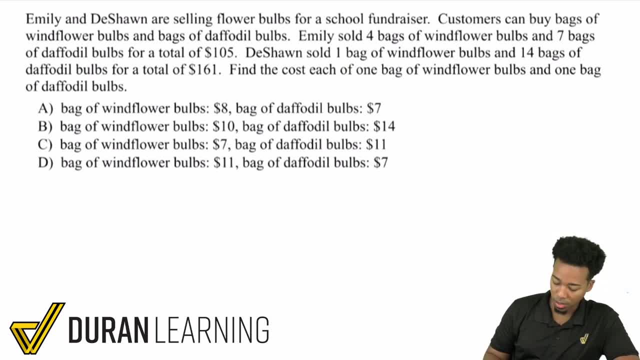 So what's the question? first, though, Find the cost. find the cost each of one bag of wind flower bulbs and one bag of daffodil bulbs Sounds good. You look at your choices. wind flower daffodil sounds great. 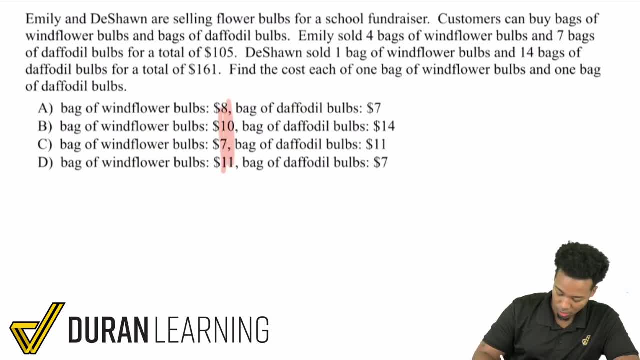 And if I check out my choices here, notice how none of these answers are the same. So if I find wind flower first, I know that I can get the answer right away. If I look at the options for daffodil, I see that these two are the same there. 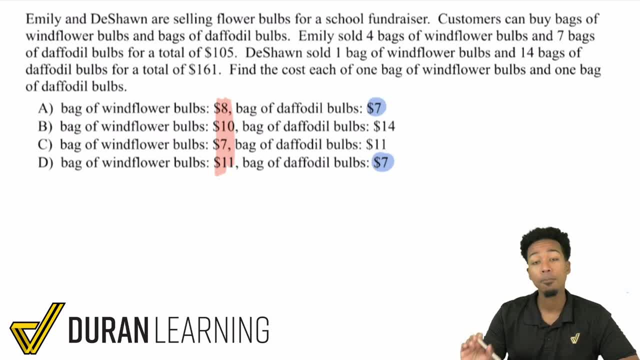 So if I get seven for daffodil, I know I'm going to have to do extra work because I'm going to have to find the wind bulb that way, Or wind flower. excuse me, Because the thing is, if you find seven for daffodil, you know that you have two options. 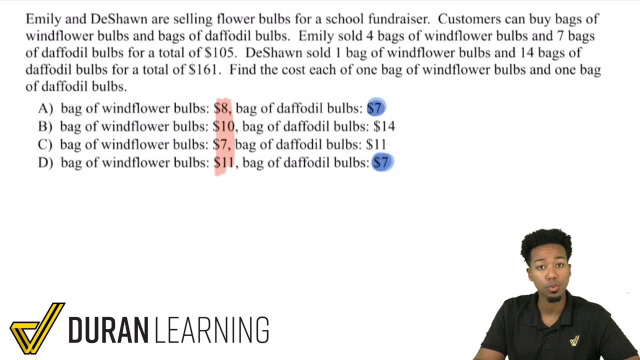 with seven for daffodil. so you're going to have to go ahead and find wind flower as well. So let's go ahead and get to work here. So we want to know the cost of each of one bag of wind flower. so I'll say W is the cost. 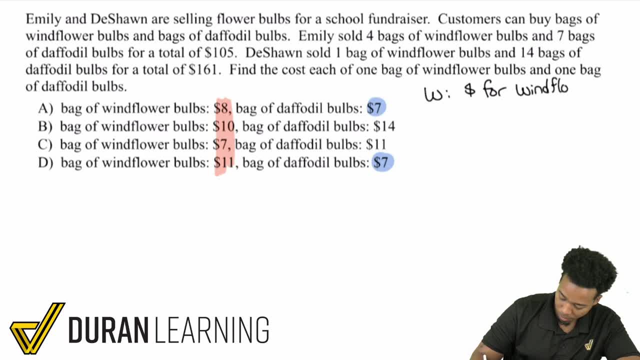 for wind flower, And then we have D for daffodil, the cost for daffodil, All right. So with that set my math part, people, let's go ahead and see what information we're given. Over here. we see that Emily and Nashawn are selling flower bulbs for a school fundraiser. Customers can buy bags of wind flower bulbs and bags of daffodil bulbs. Emily sold four bags of wind flower bulbs and seven bags of daffodil bulbs for a total of 105.. So if we're talking about Emily, well what we see? again, she sold four bags of wind flower. 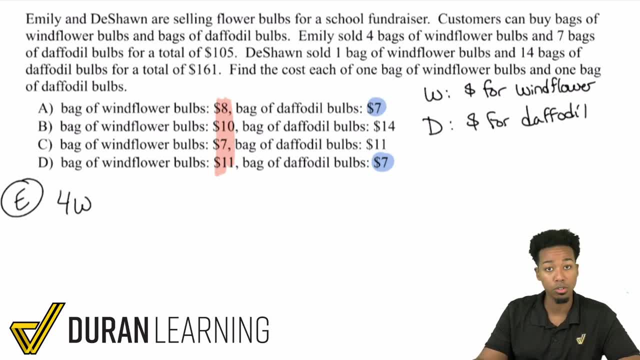 So again, to get that total cost would be four times W because W is the cost. Okay, So we add that with so over here. so, Emily, four bags of wind flower bulbs, seven bags of daffodil bulbs, total of 105.. 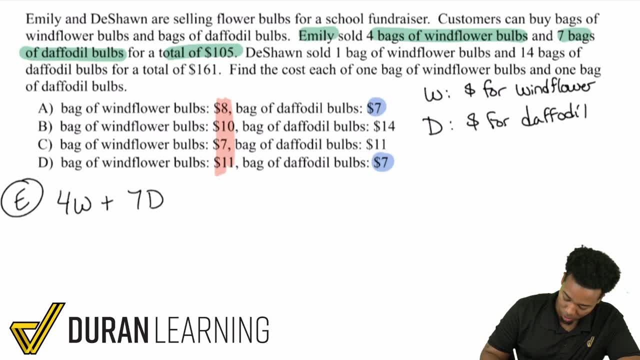 So four W plus seven D plus seven daffodil bulbs equals a total of 105.. Then over here, if we look at our friend Deshawn, one bag of wind flower bulbs, 14 bags of daffodil bulbs. 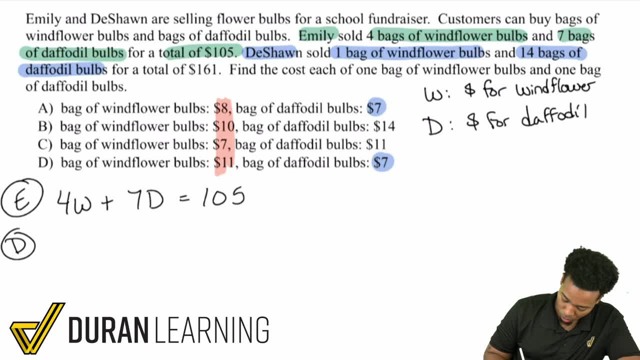 So I see over here for Deshawn we have one bag of wind flower, So just W, plus 14 bags of daffodils, for a total of $161.. So now that we have this part of people, we can go ahead and we can find a way to solve. 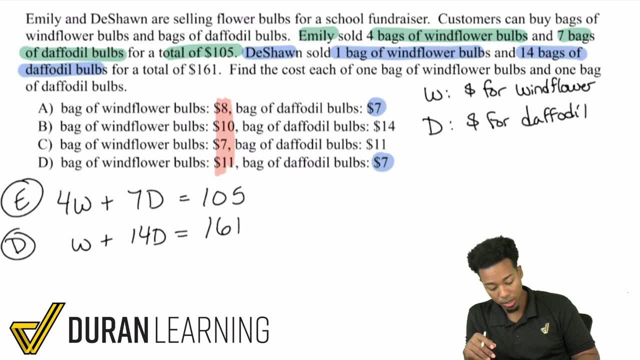 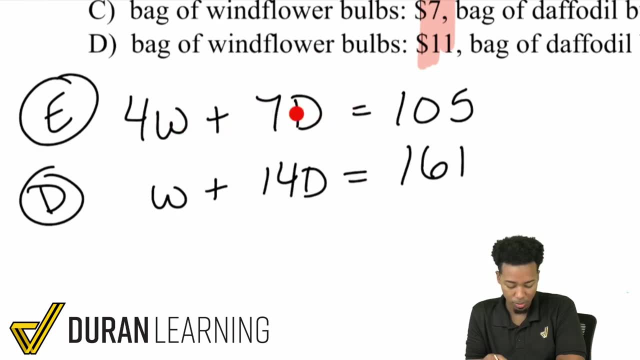 this We can find a way to solve. So let's think about the best way to solve this. I'm looking at this and I'm saying, Hey, I mean, I could very well multiply this, this equation, by two to get 14.. 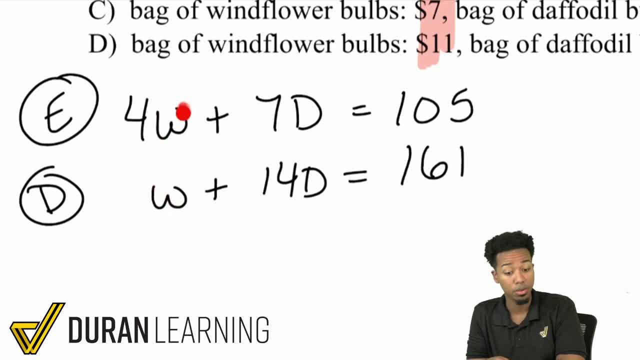 I can multiply this bottom one by four to get four on the W. You know, I could also so well, that would pretty much be it. Those are my only two options. If I wanted to do substitution, I could do substitution because I can move the 14 D to. 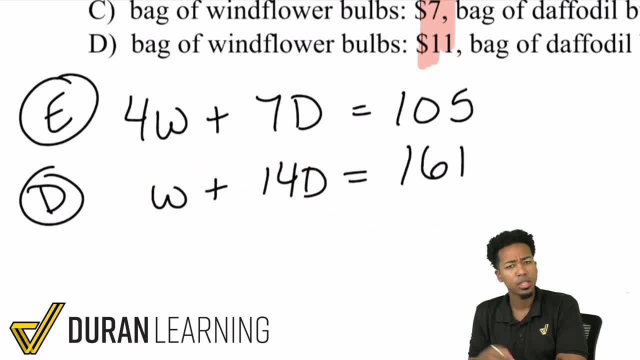 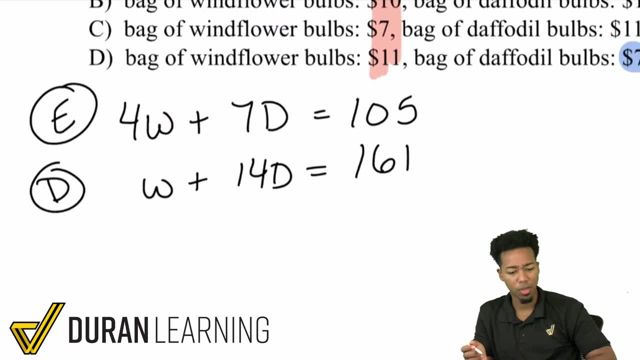 the other side to get W by itself. So I've got options here. right, We've got options, but I think the easiest way is definitely going to be just to multiply this top one by two. I'm going to go ahead and go that route. 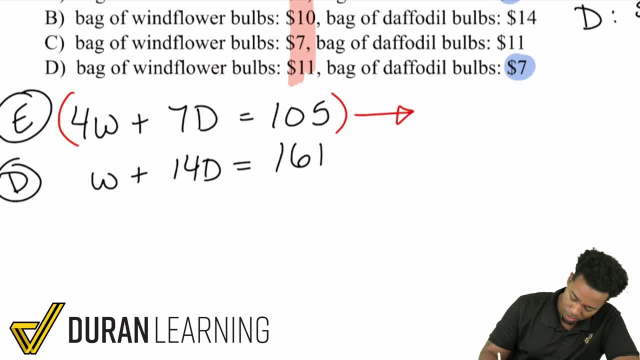 So here we go. Let's take this entire top equation, Let's multiply by two And remember: the reason that this is okay is because whatever you do to one side, you do to the other. Okay, Multiply the entire equation by two. that works. 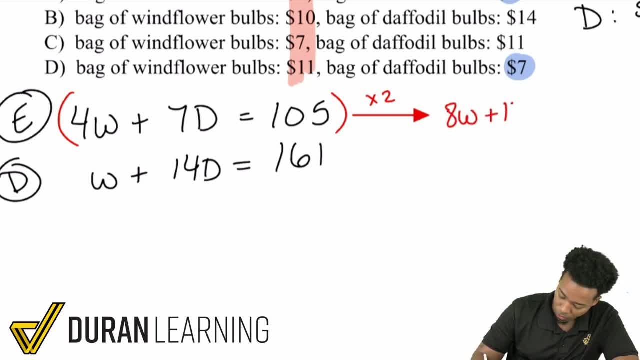 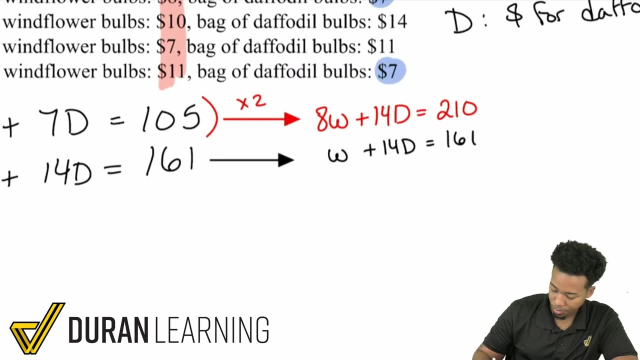 So four W times two is eight W. seven D times two is 14 D. one Oh, five times two is 210.. We will rewrite the first, the second equation, as it was no problem. So W plus 14 D equals one 61.. 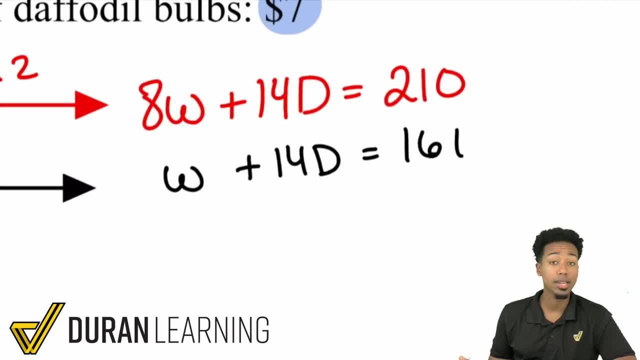 And so, checking this out over here, what I can do now my part of people is I can go ahead and subtract these equations. So right over here I'll subtract the equations. Eight W minus W will be seven W. 14 D minus 14 D cancels out. 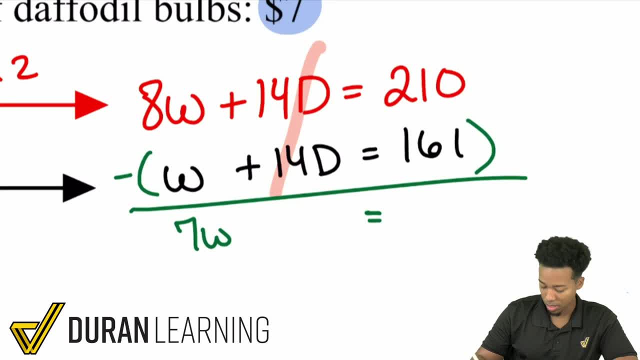 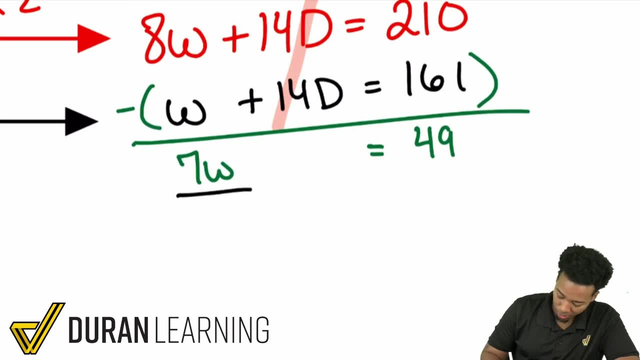 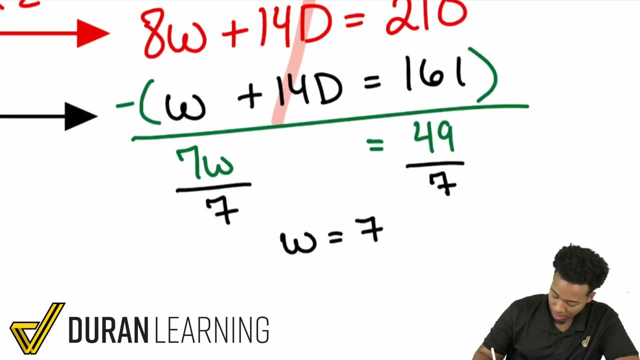 And then 210 minus 61 is going to be 49. So we have seven. W equals 49. to get W by itself, I would divide both sides by seven, giving me W equals seven, And that means $7 per wind flower bulb. 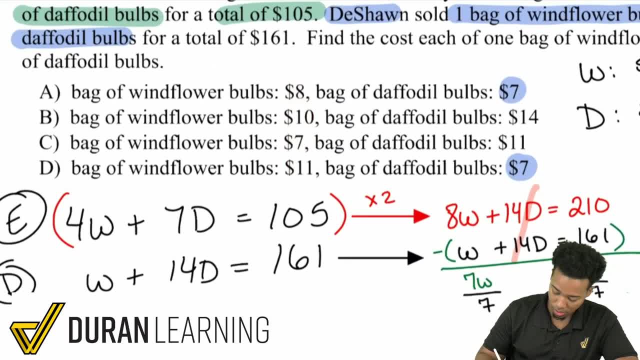 So for windflower bulbs, Where do I see seven There? it is right over here, And so my answer is C, and I'll go ahead and highlight the whole thing. That's the only question or the only option that has $7 windflower bulbs. 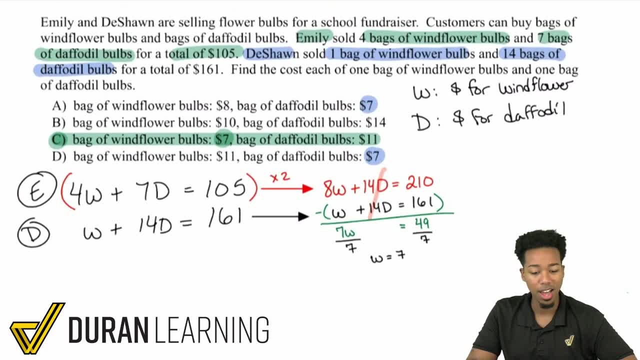 So we're good. No other work needed to be done And we can feel proud that we've done this the right way. Now let's go ahead and go into this last one on part of people. One more example here. You know I gotcha. 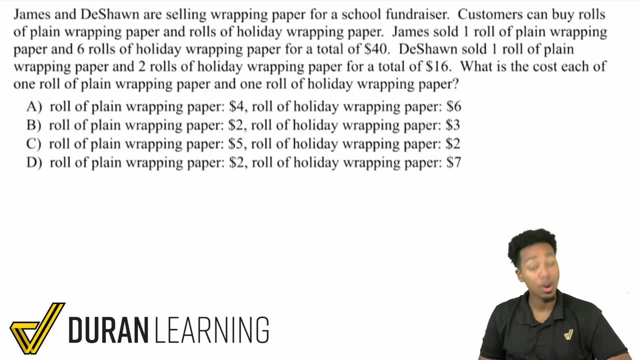 Let's talk about James and Deshaun here, And they're talking about a wrapping paper here. So look. the question here is this: What is the cost Each Of one roll of plain wrapping paper and one roll of holiday wrapping paper? 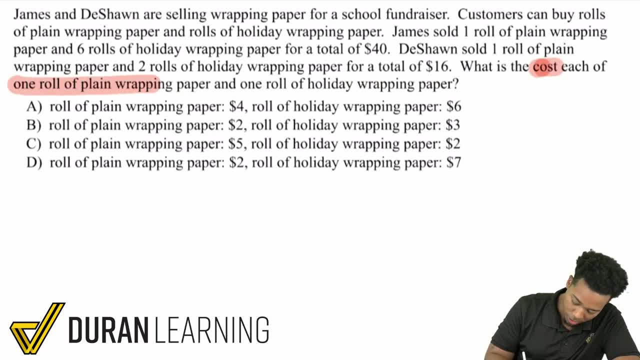 Sounds good. So the cost: one roll of plain wrapping paper, one roll of holiday wrapping paper, So boom. those are the two things we're looking for, So I'll write those down. I see that we have. we have a. let's go and say P for plane. 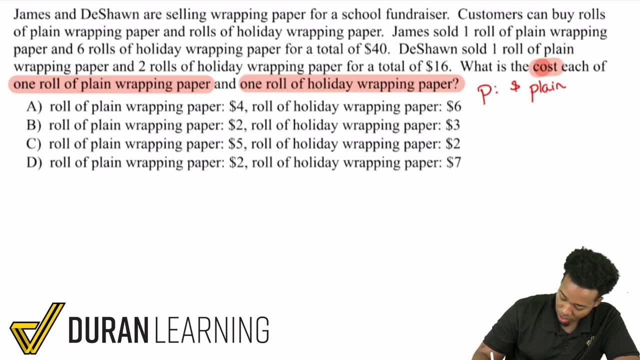 So the cost for plane, and then we have over here H, which is the cost for holiday wrapping paper. So let's see what the relationship is, Let's see what equations we can create. I see over here they're selling wrapping paper for a school fundraiser. 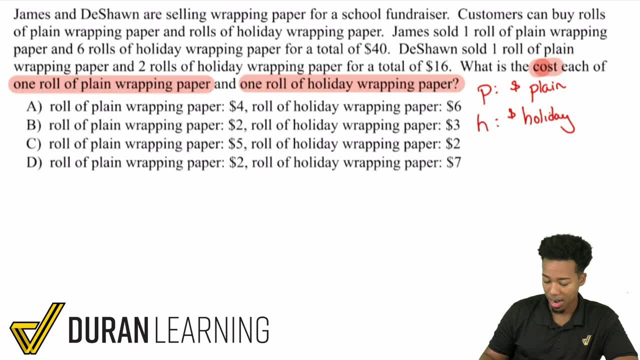 Customers can buy rolls of plain wrapping paper or holiday wrapping paper. We have that written down. James sold one roll of plain paper and six rolls of holiday paper for a total of 40.. Let's go ahead and highlight that James: one roll of plain, six rolls of holiday, total of 40.. 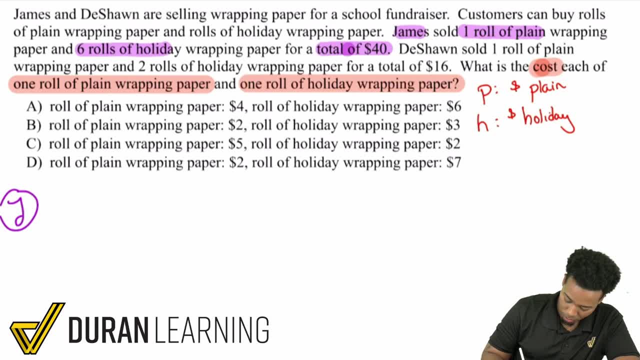 Write that out. So, James, right over here, One roll of plain, So the cost is just P, because it's just one of them. And then from there we have six rolls of holiday wrapping paper, So six H, because again the holiday wrapping paper costs H amount. 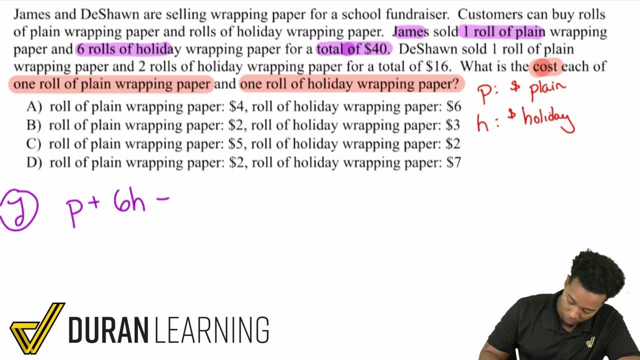 And then you multiply that by six, because it's six rolls. If you add all of that together you'll get that total of $40.. Up next we look at Deshaun: One roll of plain, two rolls of holiday- total of 16.. 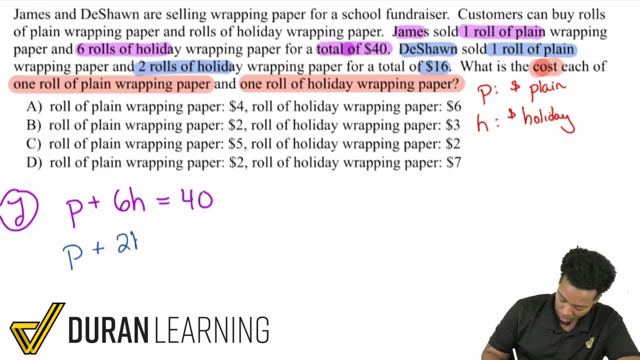 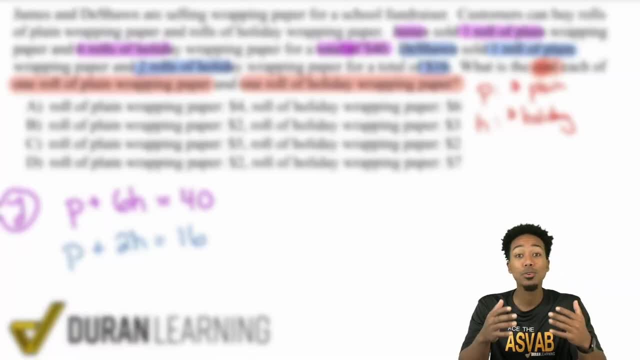 So one roll of plain, two rolls of holiday, And that was 16. And really quick. before we continue my math, party people. I know you're enjoying this And you can have thousands of problems just like this in our program. 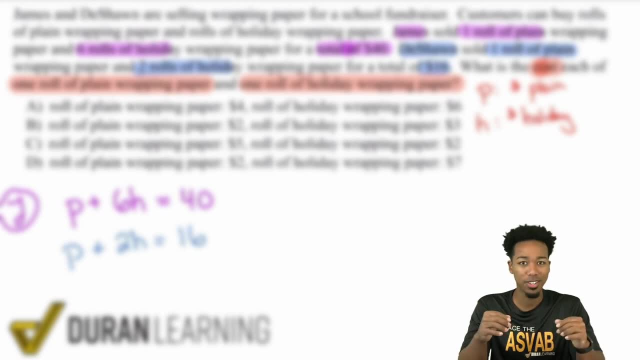 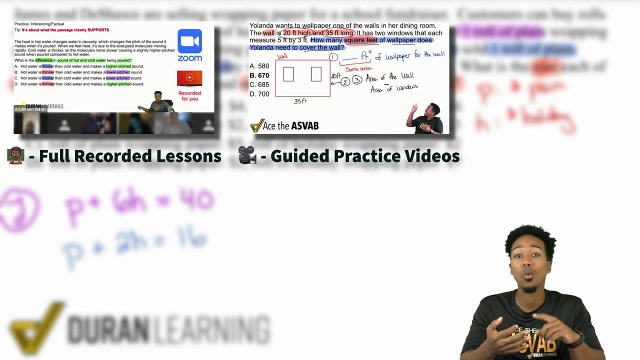 In our program you have four main things to help you succeed, and more. But mainly in our course you're going to get access to recorded lessons. You're going to get access to guided practice, just like this: worksheets that you can print out and try or keep them online. 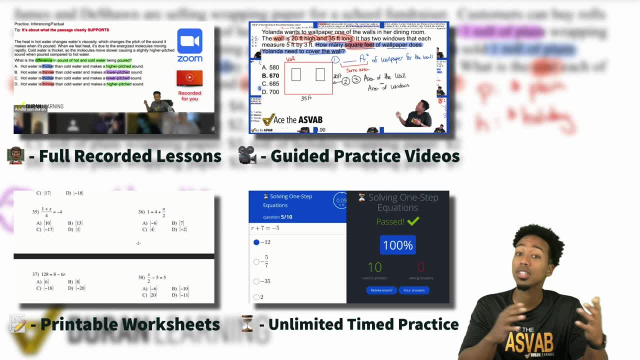 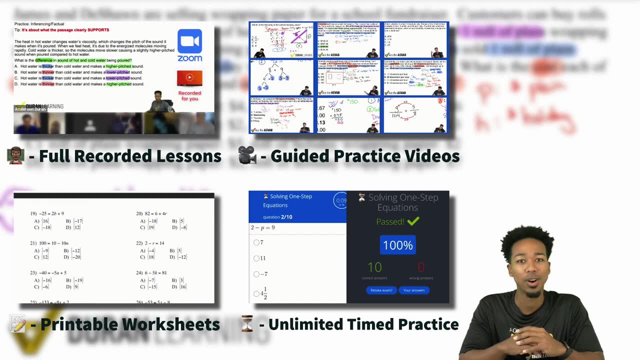 And, lastly, speed drills to raise your confidence. That way, when you take the test, there's no test anxiety, There's no pressure Because you've been timed before. You know what to do, And that's the feeling that we want. 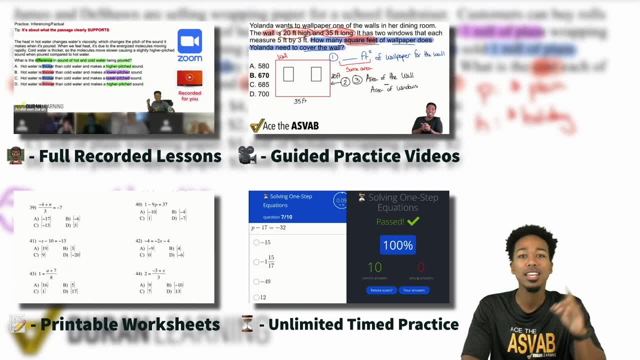 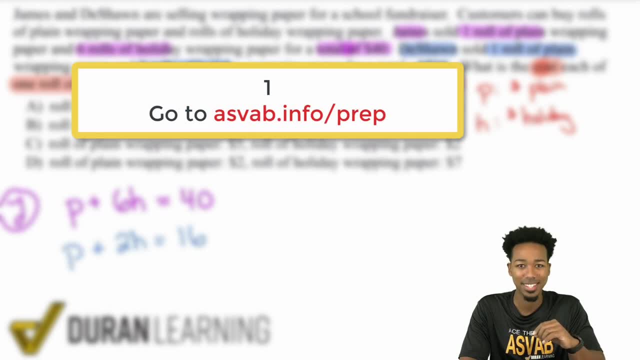 And all of that's included in our program, and more. So take a brief moment, click the link here in this video or in the description to learn about the program, and then reach out to us if you have any questions. Sign up now. Let's get going. 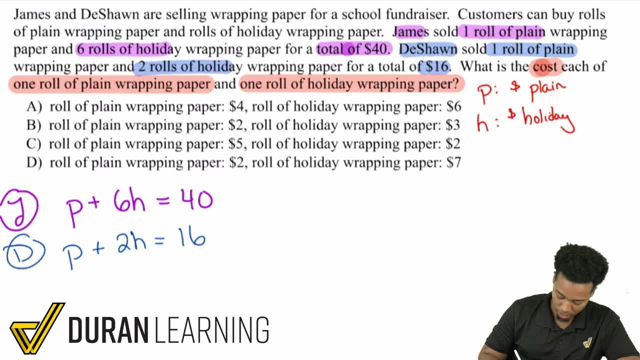 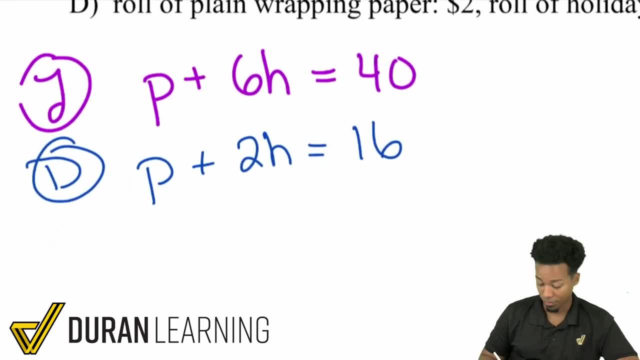 And let's get back to the problem. And so look at that, That's for Deshaun, right there. Look at how quick we can set this up once we're used to this idea, Because now what we can do- my party people- is actually very, very straightforward here. 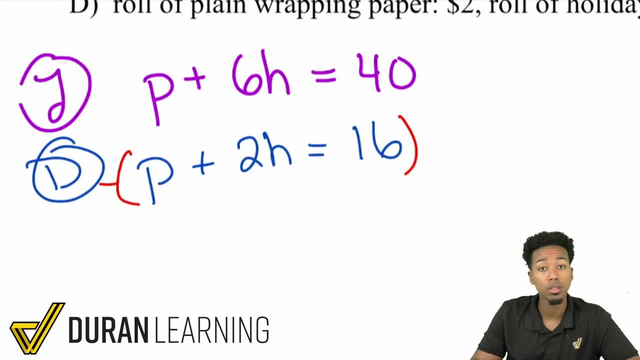 We can just subtract the equations and we're good to go. So p minus p, that's actually going to cancel out. That's going to give us a really easy time. That's going to give us a really really good, easy time here. 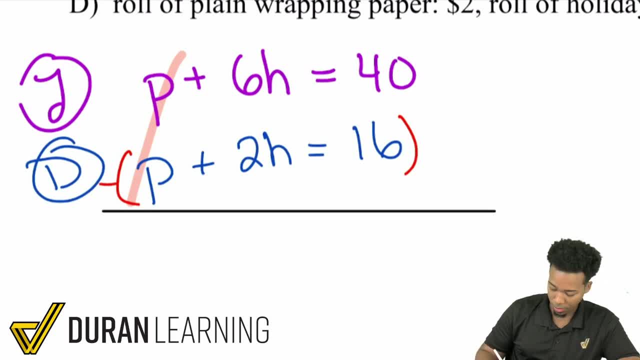 So, right there, those cancel out. Then we're going to have ourselves 6h minus 2h because again, you're subtracting. Don't forget that You are subtracting right there. So 6h minus 2h is 4h. 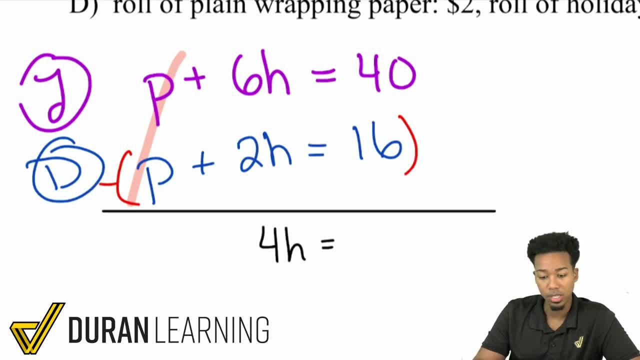 Be very careful there. And then 40 minus 16, what's that going to be? Well, 40 minus 16 is going to be what? Well, that's going to end up being 30, 24.. All right from there. we just have to solve for h here. 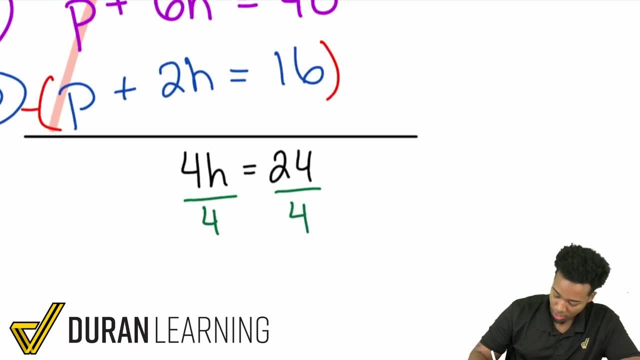 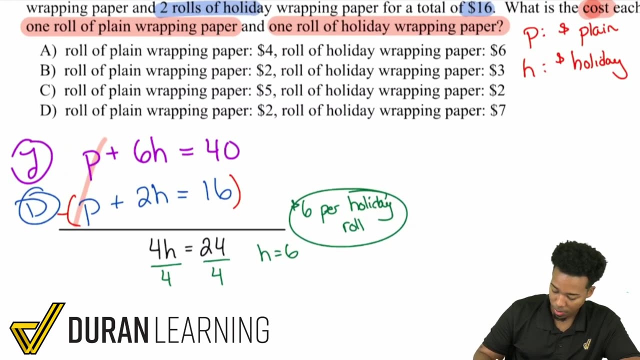 So we'll divide both sides by 4, giving us h equals 6.. So for the holiday, it's $6 per holiday roll, right there. So do we see $6 for a holiday roll? Yep, I see that right here. 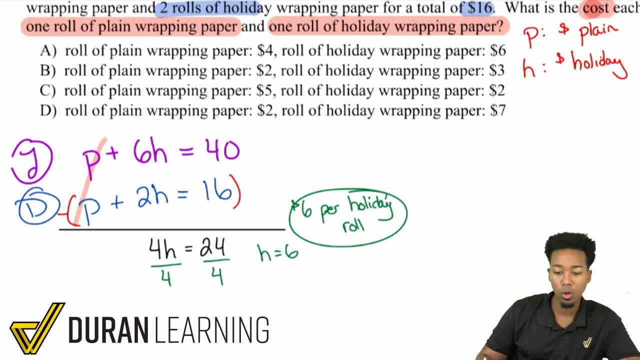 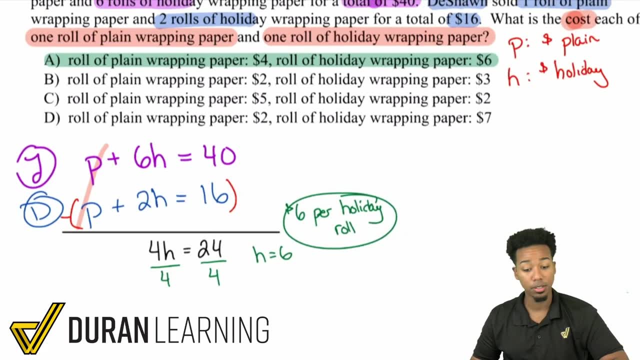 Holiday wrapping paper: $6,, then 3,, 2, and 7.. No other answers have holiday wrapping paper: 6,, so I don't need to do the extra work. I have a as my final answer and I'm good. 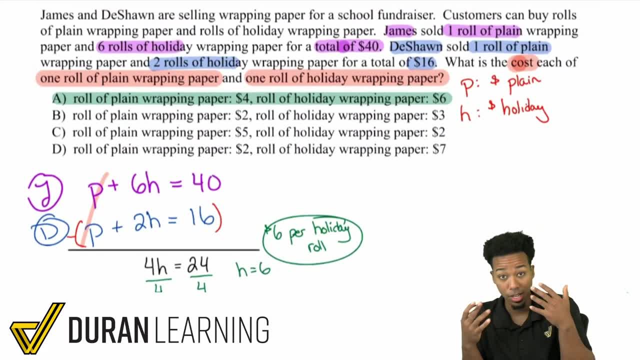 So look, my party people. at the end of the day, really, what we need to understand and fixate our attention on is being able to set up a problem, because we've been learning how to solve all the way through. And if you haven't had the chance to solve systems, well, we need to go back into those. 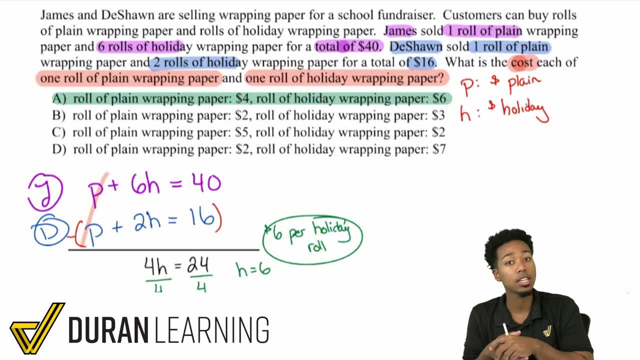 previous videos. But what you're going to do up next is you're going to look at any other guided practice videos that we have for word problems, for systems And then try those worksheet problems out and then from there do the speed drills. 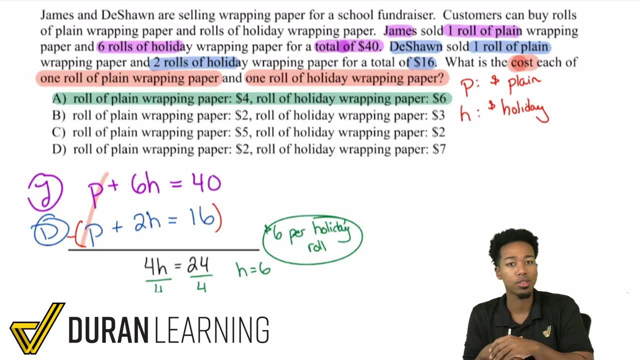 I want to see you succeed, my party people And so being able to set these problems up as quickly as you can, that's the most important task, And then, from there, solving them, that's the best. So, with that said, my math party people, I'm Anderson, your math coach. 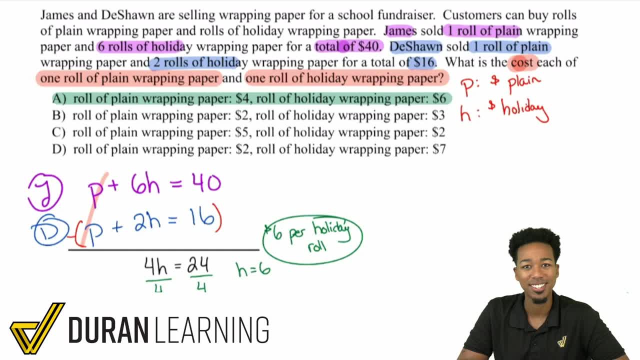 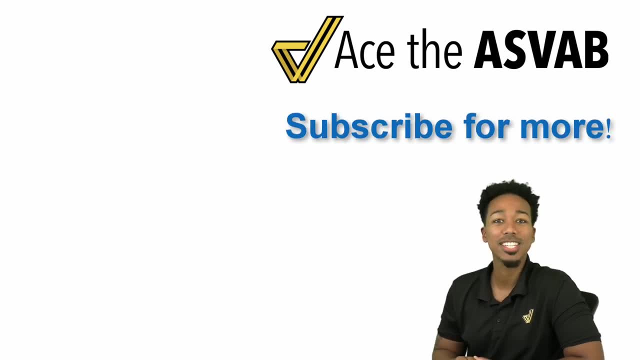 Let's keep it going the right way, Keep partying and let's raise that score. I'll see you soon And, as always, my party people, thanks for watching. You can subscribe with that button right there And you can also see a link to a video. 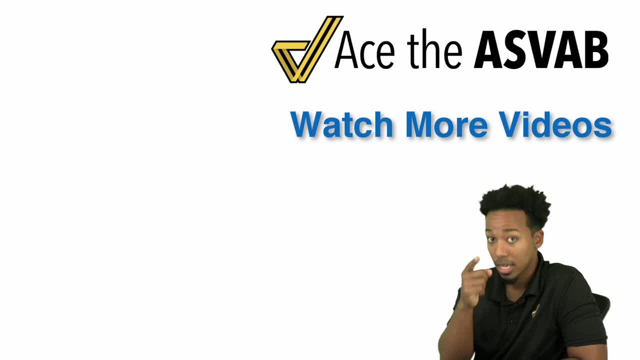 I'll see you soon. I'll post a video, just like this one right up there. But, most importantly, if you want the program and you want to raise your score the right way, every step of the way, with my support- there's that link at the bottom left.